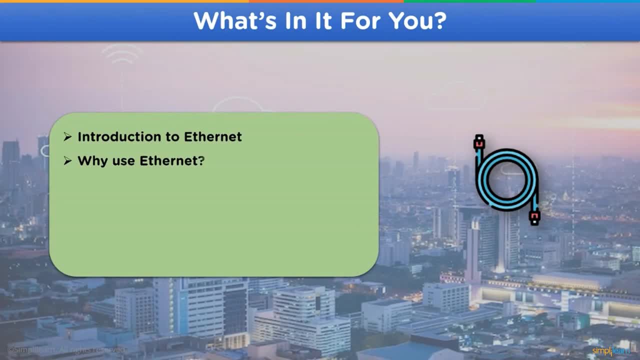 To begin with, we will look into what is Ethernet. Moving on with seeing what is the use of Ethernet, different types of Ethernet and looking into the working of the Ethernet cables. Advantages and disadvantages of using Ethernet. And lastly, difference between Ethernet and Internet. 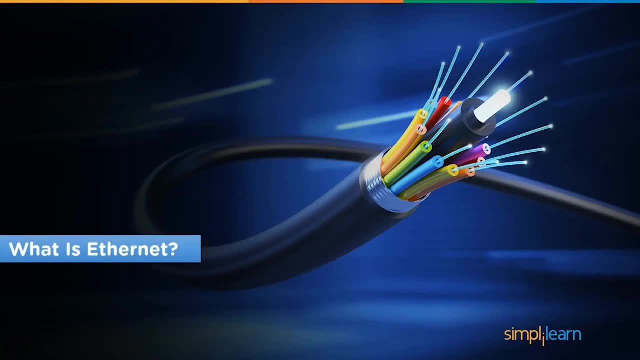 Now let's look into the first heading. What is Ethernet? 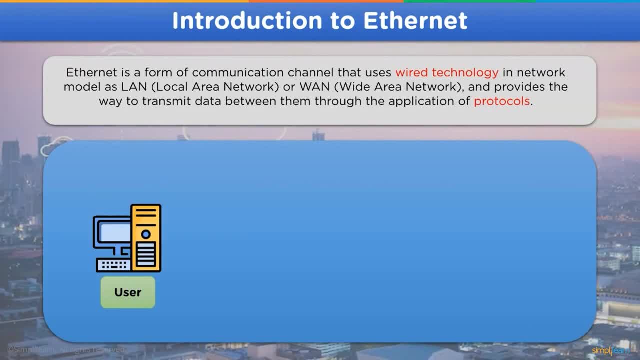 Ethernet is a form of communication network that uses a wired medium to connect devices for data exchange in a network. 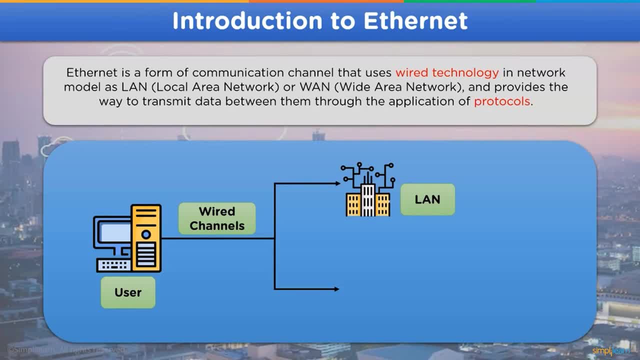 For example LAN, also known as Local Area Network. Also, WAN. 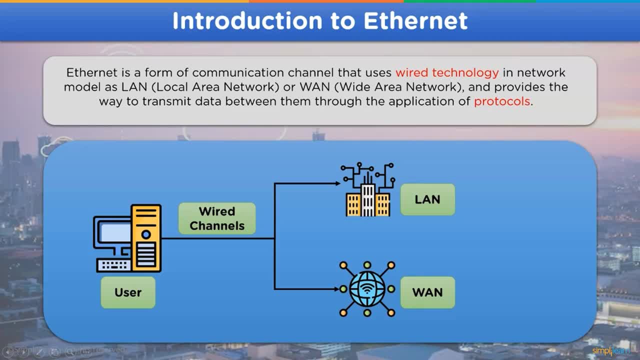 Ethernet also applies different protocol on the data to be transmitted over the communication channel efficiently and smoothly. 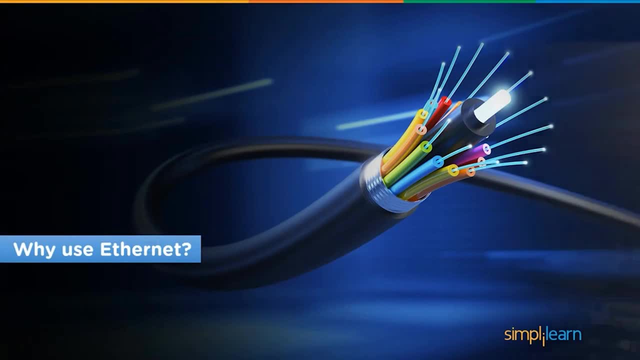 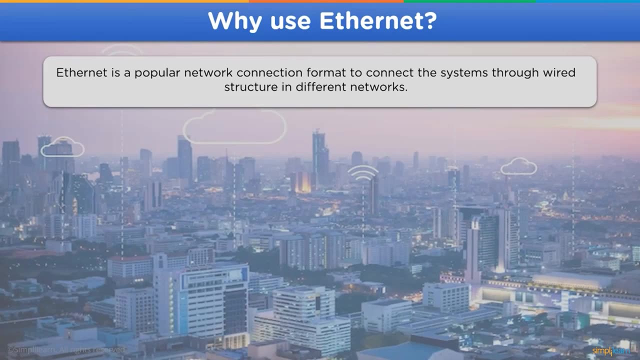 Moving on, let's look into why to use Ethernet. As we now know, the Ethernet is a mode of connection for multiple devices to share and exchange data. 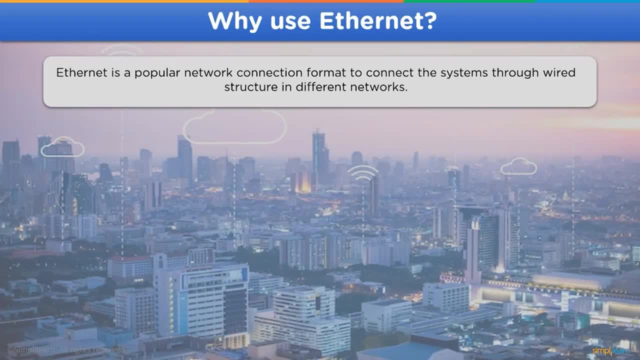 But using this way of transmission also has its benefits. For example, the Ethernet network provides us with a high speed connection for sharing data. 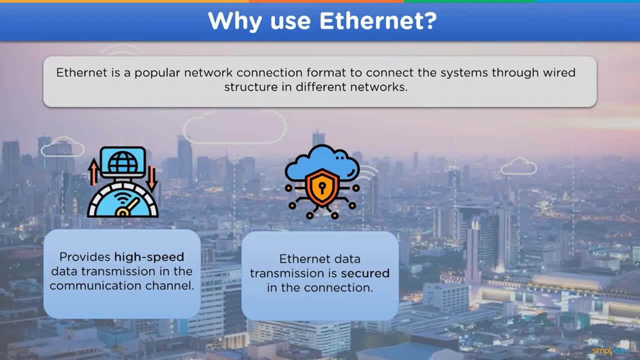 Ethernet also provides the user data with a secure channel for transmission. The data that is transmitted over the Ethernet channel is reliable and has rarely faced any issues at the sender side. Let's move on to the next heading. Now we will look into the second heading. What is Ethernet? What is Ethernet? 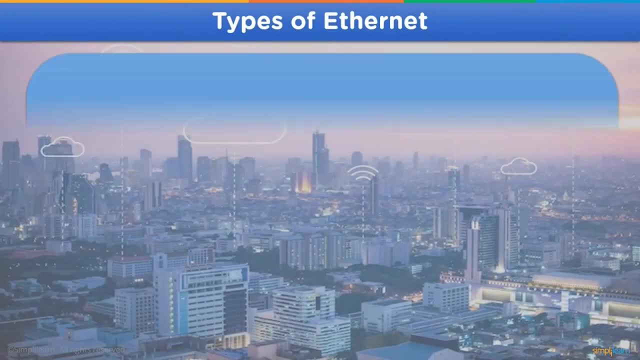 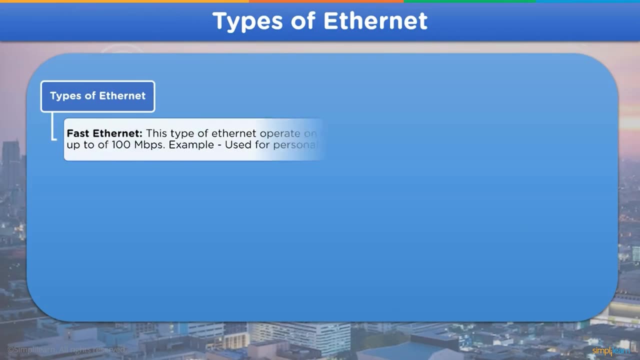 Let's first look into different types of Ethernet. In general, the Ethernet is divided into three different types. First is the fast Ethernet. This type of Ethernet operates on a twisted pair cable with a data transmission speed of up to 100 Mbps per second. 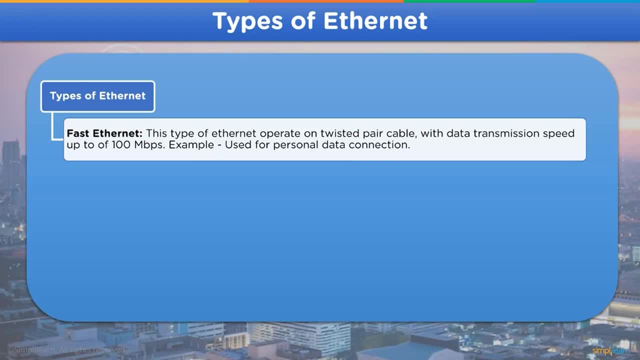 Fast Ethernet connections are used for personal connections or used in companies that require low internet connection. 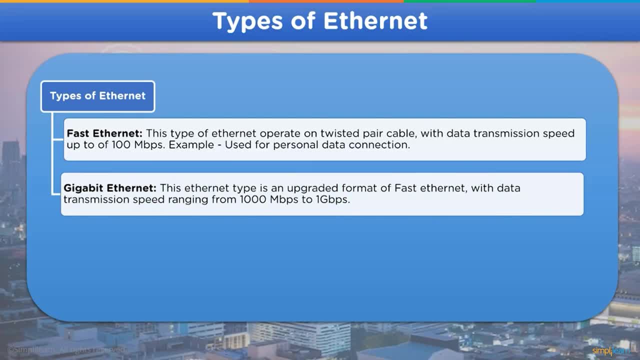 Moving on, we have Gigabit Ethernet. This type of Ethernet is used for high-speed internet connection with a speed ranging from 1000 Mbps to 1 Gbps. 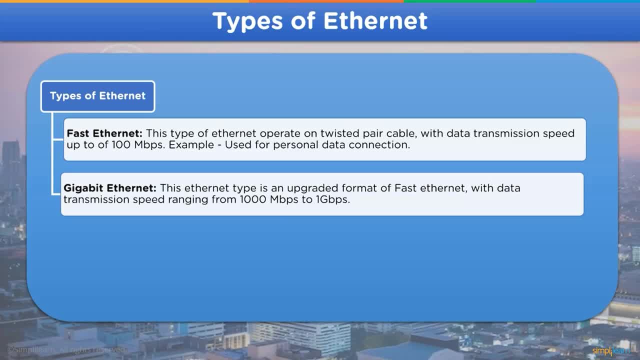 It is an upgraded form of fast Ethernet. 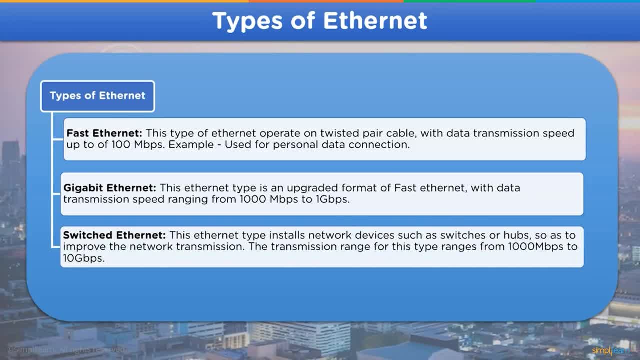 And the last type is Switched Ethernet. This Ethernet type installs network devices such as switches or hubs so as to improve the network transmission. The transmission range of this type of Ethernet is 1 Gbps per second. 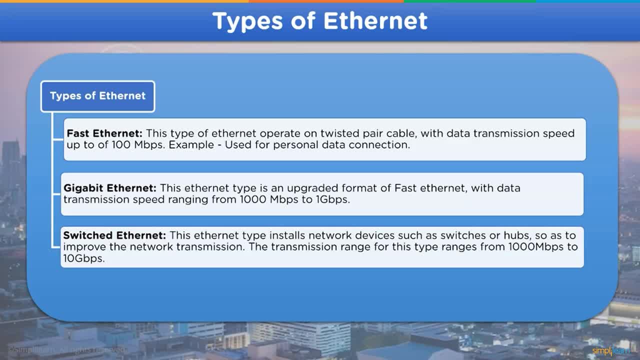 The transmission range for a switched Ethernet connection is around 1000 Mbps to 10 Gbps. 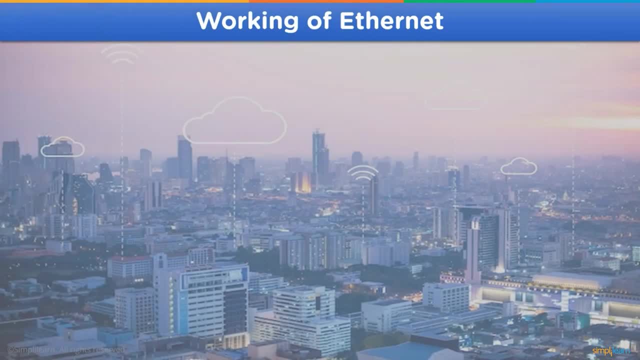 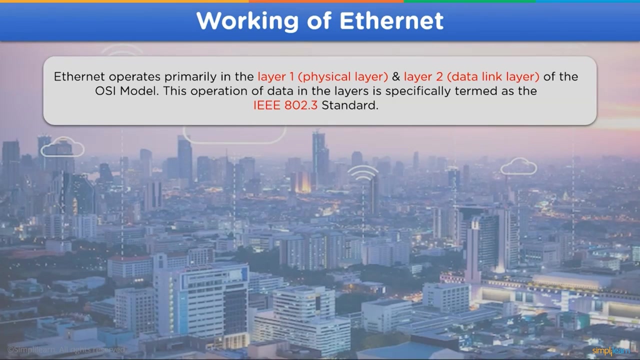 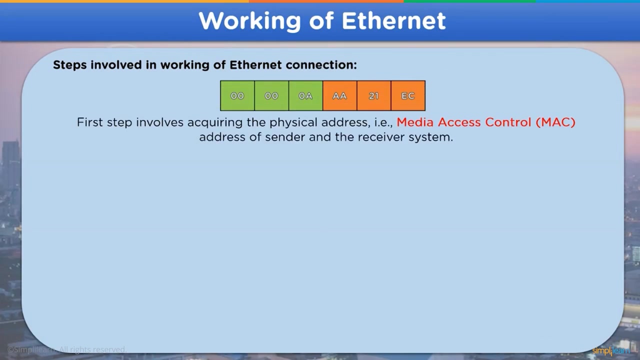 Now let's look into the working of Ethernet. Ethernet services specifically work in the first layer of the OSI model that is known as the physical layer and the second layer of the OSI model, also known as data link layer. Functioning of the Ethernet can be divided into three layers. First step being acquiring the physical address that is MAC address, media access control address of the sender and the receiver device. 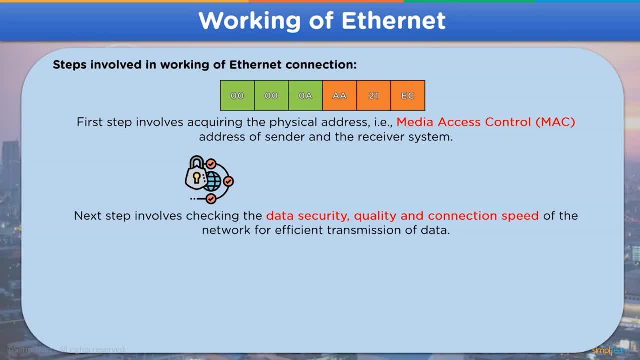 Then the second step is to check the data security, quality of the data and the connection speed of the transmission channel for efficient and smooth transmission of data over the network. 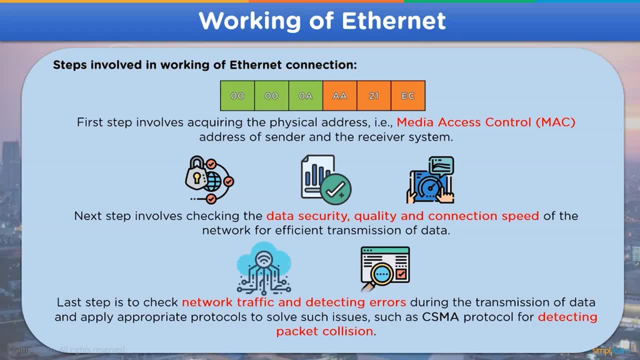 And the last step is to check network traffic. This is the first step. The second step is to check the network traffic and detect any error that occurs in the communication channel. 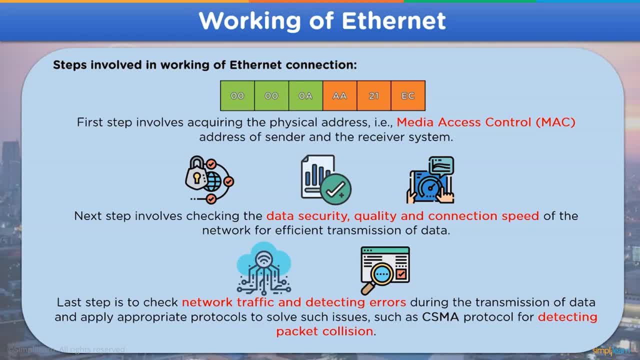 To solve these issues if occur, CSMA protocols and other protocols are used. For example, the CSMA protocol is used in case of packet collision in the network channel. Now let's look at a simple Ethernet model for further clarification of the steps. But before we begin with the model. 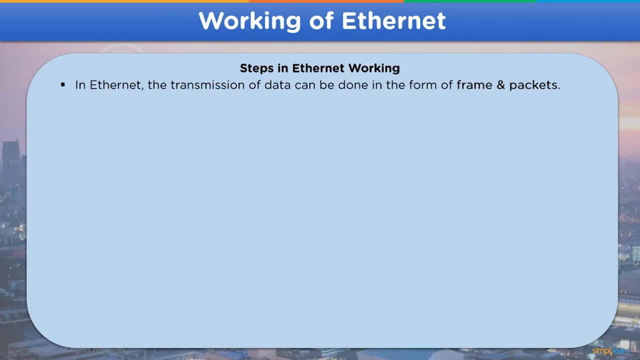 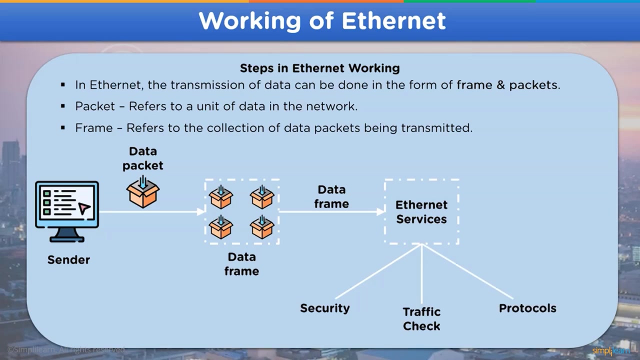 The point is that the Ethernet is a very simple model. The Ethernet is a very simple model. The point to be noted is the transmission of data over the Ethernet channel is divided into two parts. Frames and packets where packets represents a unit of data in the network whereas frame refers to a collection of data packets being transmitted over the channel. And the application of Ethernet services which includes security, traffic check and protocols being applied. The input value is the traffic data in the Ethernet channel. The output value which comes from the internal OS is the speed of theoxy-cd and the output value is the transmission times. The data transfer speed of the data on the data is the speed of the word and the data 액 on the data and that is when it reaches the receiver end. 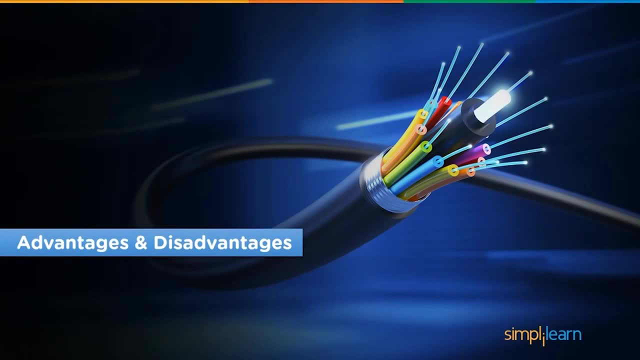 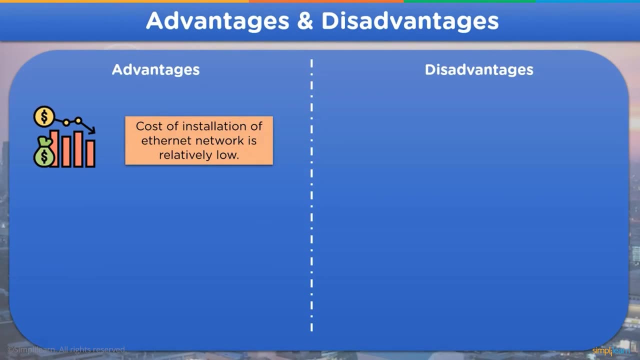 Moving on, let's look into advantages and disadvantages of using Ethernet. For advantages we have, the cost of installing Ethernet connection is low in comparison to other network channels. The security of the data being transmitted over the Ethernet channel is maintained. 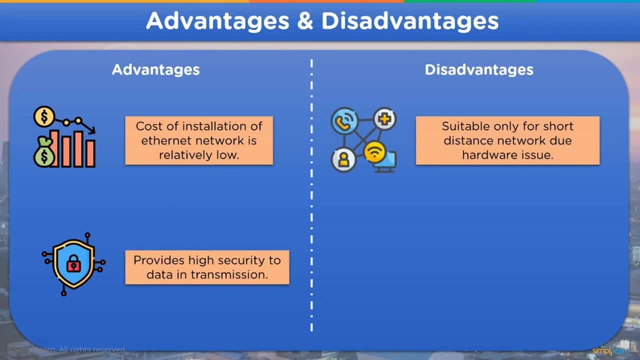 As for disadvantages we have. It is suitable only for establishing short-distance communication network due to high requirement of hardware resources, whereas Ethernet is also not suitable for sharing real-time data and information. 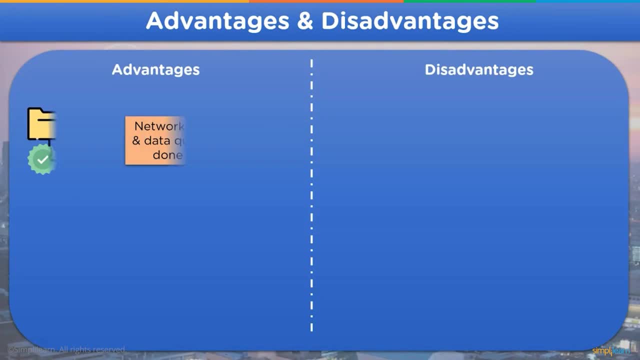 Let's look into some more advantages and disadvantages. Ethernet is suitable for maintaining the data quality of the information being transmitted. It also provides high-speed data transmission option for the network. 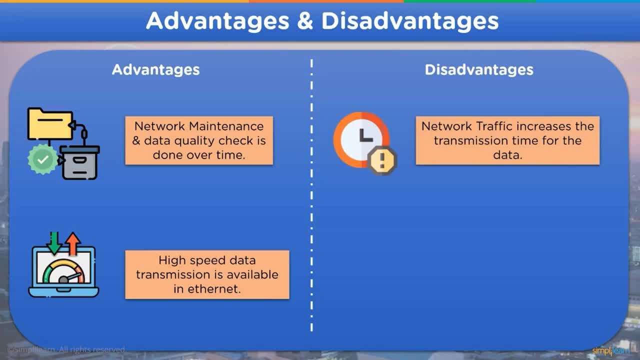 For disadvantages we have, the network traffic issue is a drawback of installing Ethernet cables. 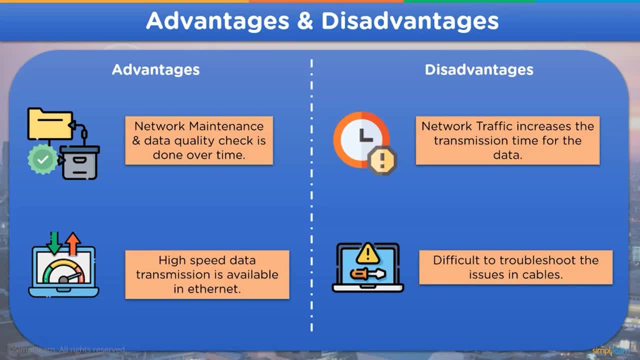 Troubleshooting faults and issues in the Internet cable is also a troublesome work. Now let's move on to the last heading for this topic. 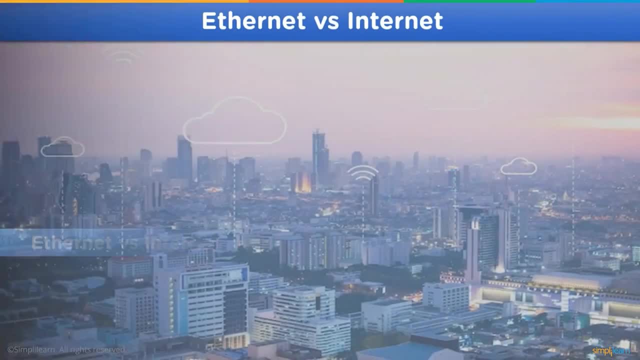 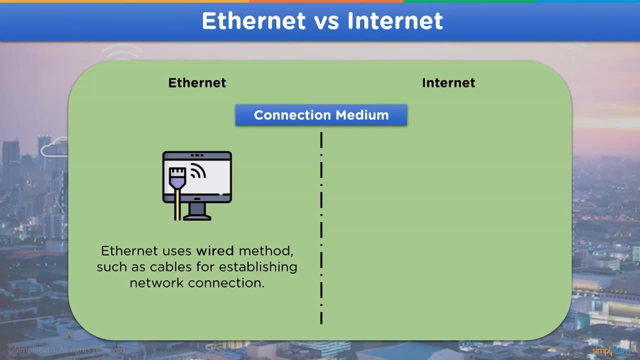 That is Ethernet versus Internet. The first difference is connection medium. For Ethernet connection, physical cables are required. That means it uses wired medium for connection, whereas in case of Internet, it uses wireless medium such as satellites as a connection medium. Moving on, the next difference is network model. The Ethernet is available only for a low-distance connection, for example LAN, whereas Internet is available for all the network connection distances, be it LAN, MAN or WAN. 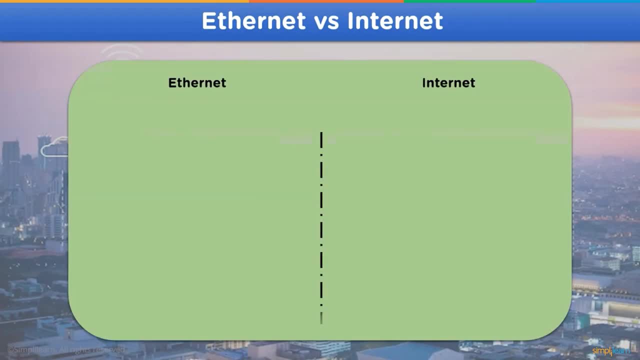 Let's move on to the next difference, that is network control. 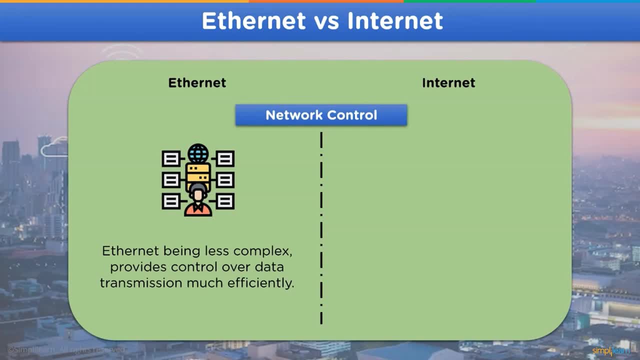 For Ethernet, the complexity of the connection medium is low. Due to the less distance it uses, and also provides much efficient transmission of data 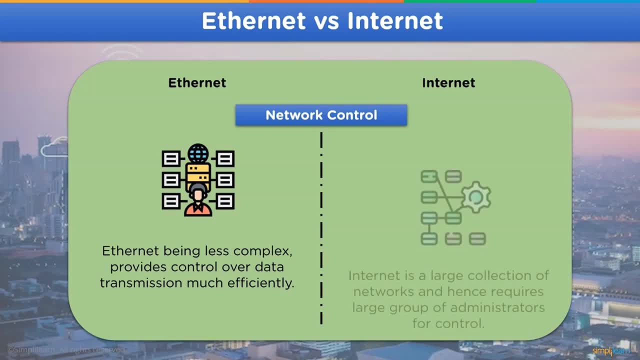 over the communication channel, whereas for Internet, is a large collection of networks and hence require large group of administrator for control. 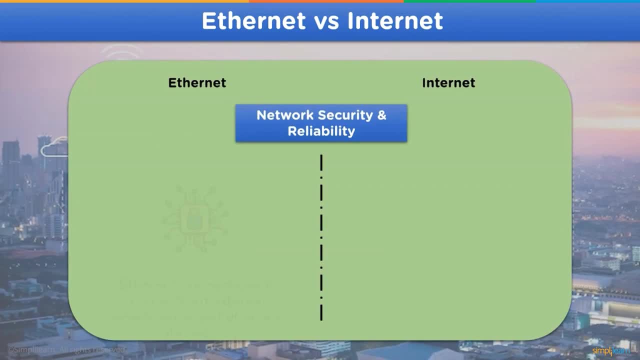 The last difference between Ethernet and Internet is network security and reliability. Ethernet connection is a secure network from external sources. Ethernet connection is a secure network from external sources. Ethernet connection is a secure network from external sources. 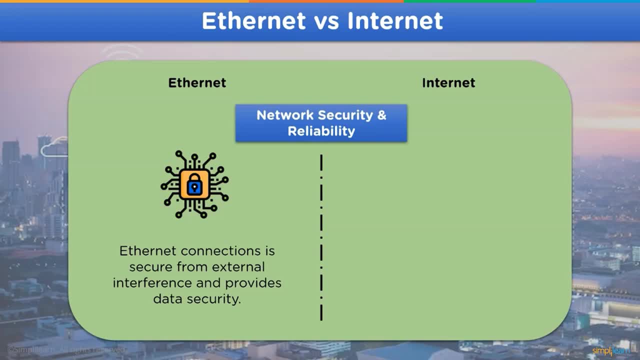 Ethernet connection in the network provides data security, whereas in case internet is an open type of connection, which is neither good nor bad, so it is more prone to hacking attempts and less secure network. 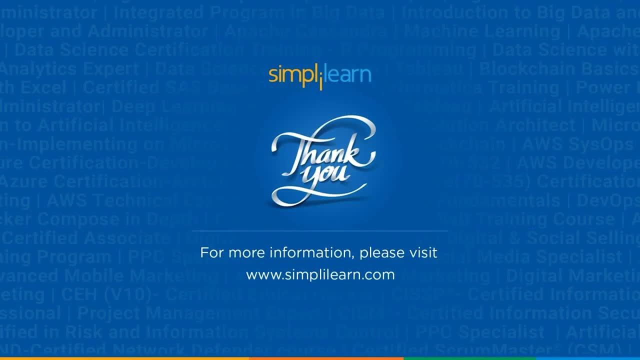 With this, we have reached the end of the video. 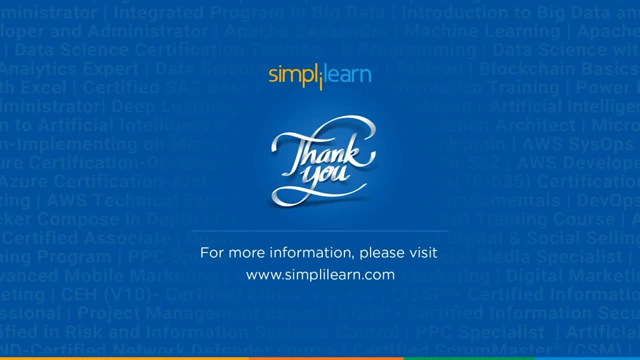 If you have any questions regarding the topic, you can ask them in the comment. Thank you for watching. Once again thanks for watching. Thanks for watching. 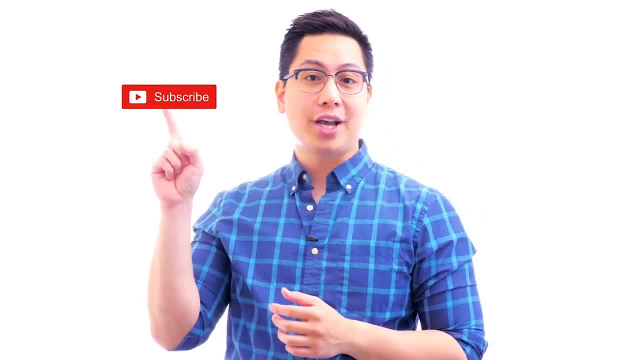 Hi there, if you like this video, subscribe to the Simply Learn YouTube channel and click here to watch similar videos. To nerd up and get certified, click here.